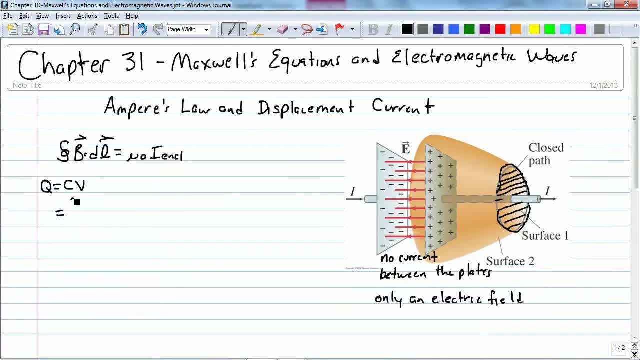 case parallel plate, it's the easiest for us to use. that's just epsilon naught times the surface area of the plate divided by the distance, and the potential is just the electric field times the distance between the plates. so if I simplify, these are going to cancel and I have epsilon naught a times e, but 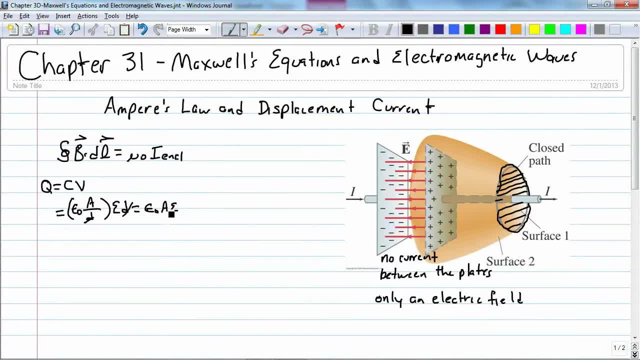 the electric field times. the area is just equal to the electric field times. the area is just equal to the electric field times. the area is flux. Now I'm going to have this current I call a displacement current. It's been found that this is actually a bad term. There is no current that flows, but this was something. 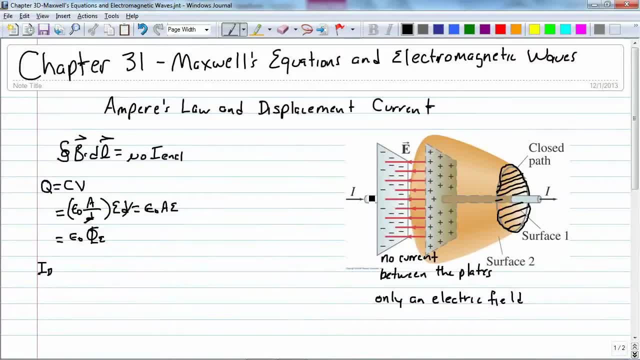 that Maxwell modeled. They thought there was some kind of unknown current that flowed in between these plates, but it's been found that it doesn't happen. But they still use this term, displacement current- And that's just going to be equal to the derivative of 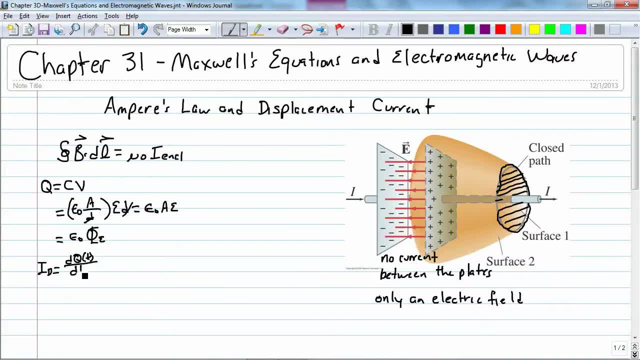 the charge with respect to time on the plates And that is just going to equal. well, if I take the derivative of the the left-hand side, I can take the derivative of the right-hand side and that's just the derivative of the electric field flux. And now I have a new enclosed current that I can.